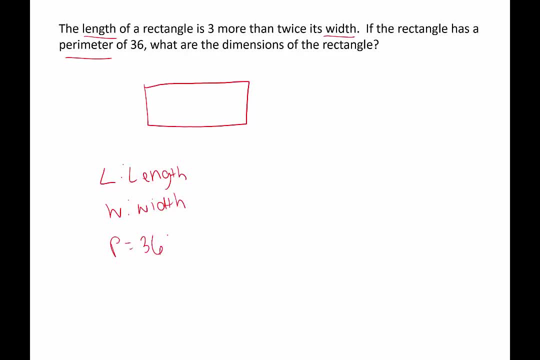 We know the perimeter is 36,, but it would also be helpful if we knew the formula for the perimeter of a rectangle. So you might recall that the perimeter of a rectangle is 2L plus 2W, And we want to know the dimensions of the rectangle. 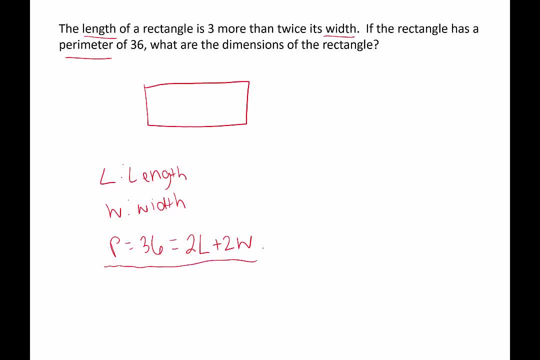 So what we're looking for is: we're going to look for this and we want to figure out the values for L and W. In that first sentence, the length of the rectangle is three more than its width. So three more than implies something plus three. 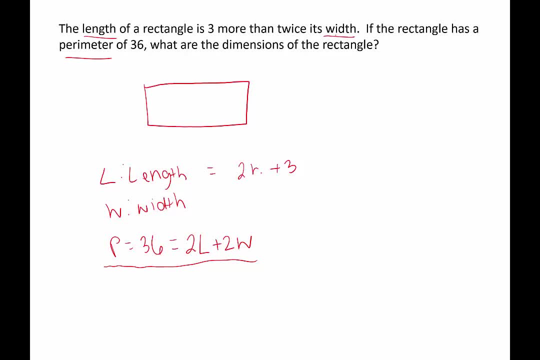 And then twice its width, that would be two times W. So the length is two times W plus three, which I'll put here: two times W plus three, And the width is W. So what I'll do is I'll take these dimensions up here and I'll plug them into the perimeter formula that we have at the bottom. 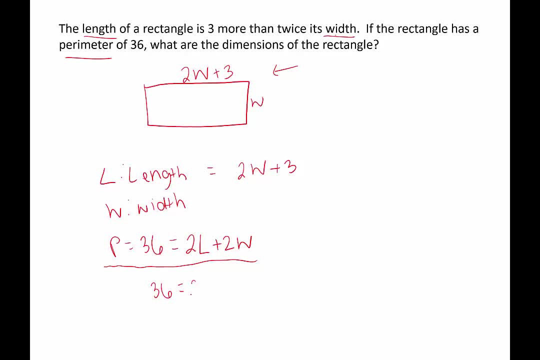 And we'll use 36 instead of P, just to get rid of a variable. And then, instead of L, we're going to use 2W plus three, and then plus 2W, And now we're down to just one single variable. 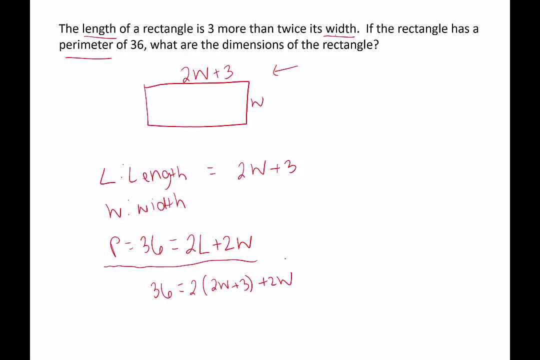 We'll clean up the equation and then figure out the value of W first, And then we'll be able to figure out the value of the length as well. So this is 36 equals 4W plus 6 plus 2W. I'll combine like terms: 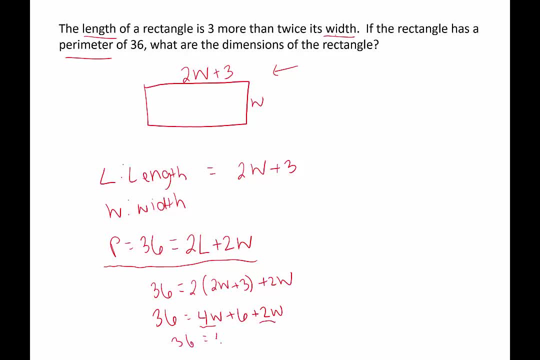 4W plus 2W is 6W. 6W plus 6, subtract 6 from both sides And we get 30 equals 6W. Divide both sides. Divide both sides by 6. And we get 5 is equal to the width. 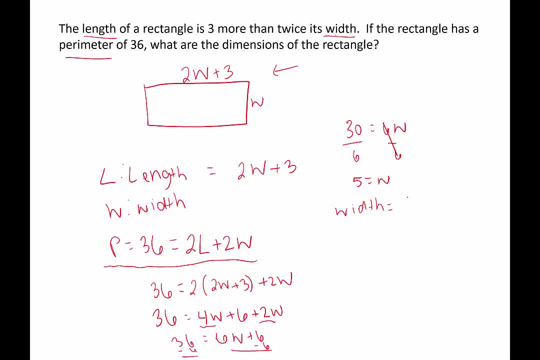 So now we know the width is 5, but it asks us to find the two dimensions. So we'll figure out the length by plugging 5 in for W, back in this expression that we had to represent length. So that would be 2 times 5 plus 3.. 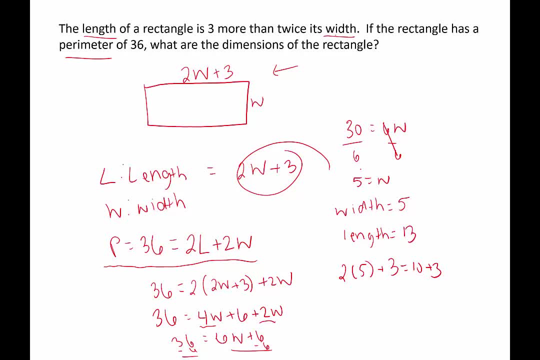 That would be 10 plus 3.. The length is 13.. Now I feel pretty good about these numbers, but I like knowing for sure that I'm right. So one thing that I can do is I can make sure that if I did the perimeter calculated, the perimeter based on this width and this length.